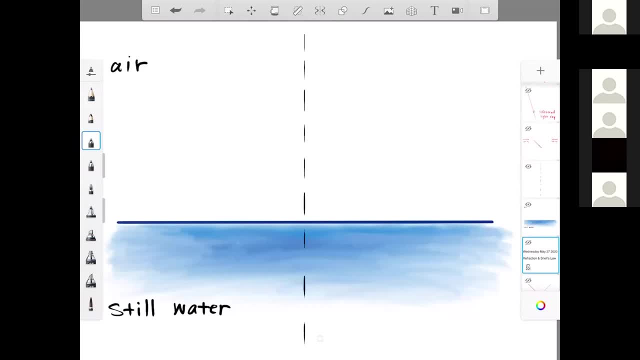 water. First, let me draw a line that is perpendicular to the surface. From this point on, I'm going to call it normal to the surface. Okay, so just to be clear: when I say normal to the surface, that means perpendicular to. 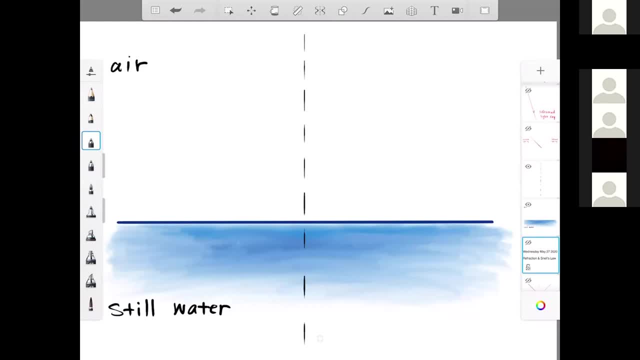 the surface Anyway. so we know from the law of reflection right that if we were to shine some light onto a shiny surface- like water is definitely shiny- some of that light will be reflected at an angle that is exactly equal to the angle in which light came into it. 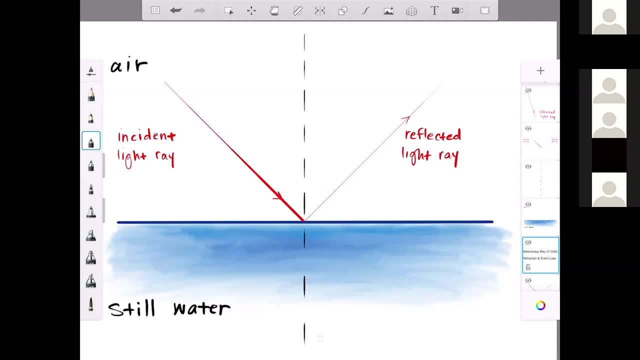 All right, that's the law of reflection. Now, normally, when you're talking about a perfect specular reflection, all of the light gets reflected, But in the case of something like this, that's not really what happened. So you got some of the light coming in some. 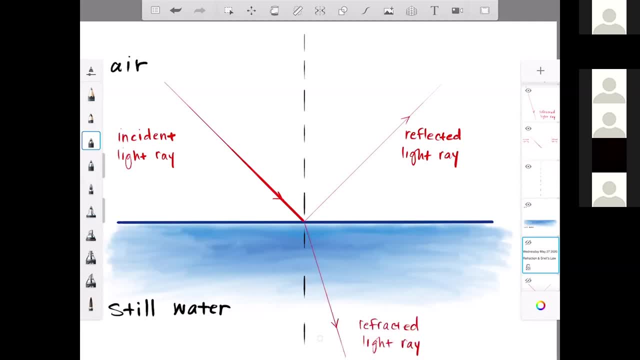 of it gets reflected and then the rest of it ends up getting refracted. So refraction means light gets bent through the surface. Okay. So when it travels through some sort of material, okay, it gets bent. So we have a couple of. 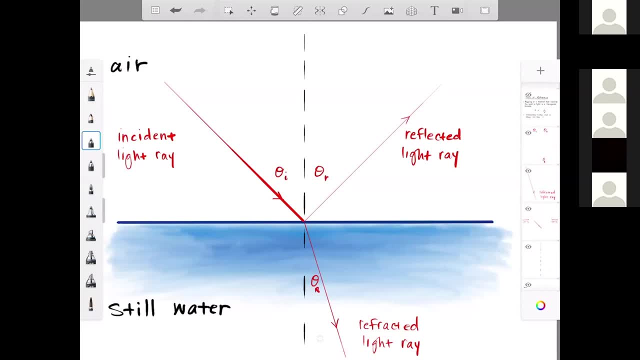 angles. here Theta i is the angle of incidence, So the angle in which the light ray comes in with And we always measure it to align normal to the surface, And we know from last time- not last time but the time before last- that the light is coming in at a certain angle. 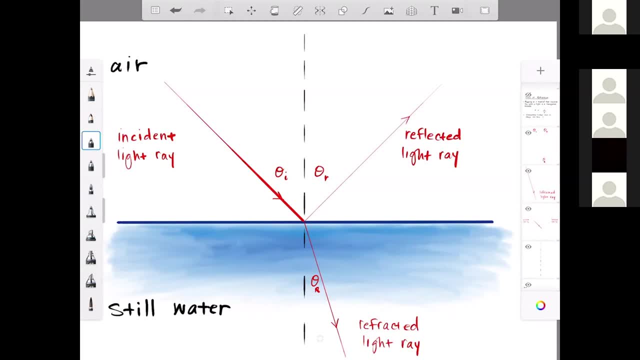 Of course, if you're looking at the video, you're going to see that the angle of incidence has to be exactly equal to the angle of reflection. That's, of course, the law of reflection. But now we have another angle called the angle of refraction. So since both of those things 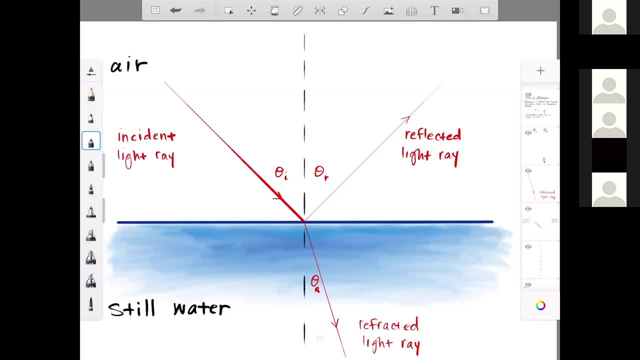 start with the letter R. I use the capital R in the lowercase r, So Theta capital R is going to be the law of refraction, For now at least. Now, how the light gets refracted is going to be dependent on the angle of incidence And for now at least, we'll use 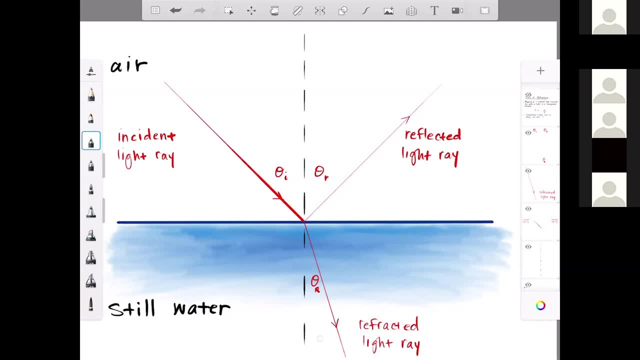 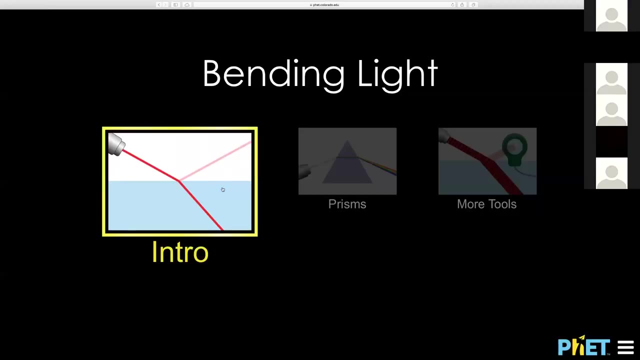 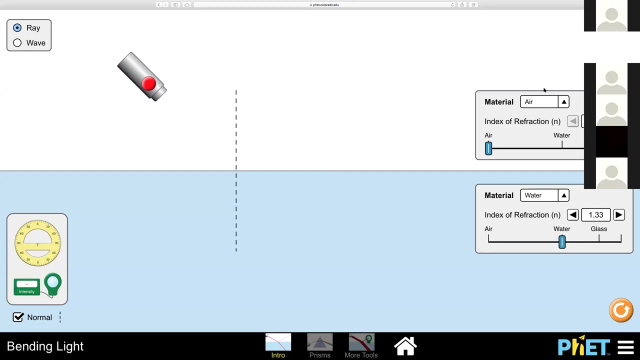 the angle of incidence, And just the angle of incidence has to be exactly equal to the. upon what type of material is the light going through? So now let me share with you another screen to give you a better idea of how this works. So I hope you guys can all see this. It's a similar drawing to what we had on the. 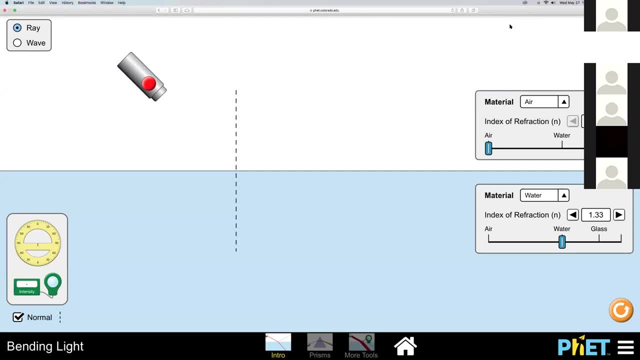 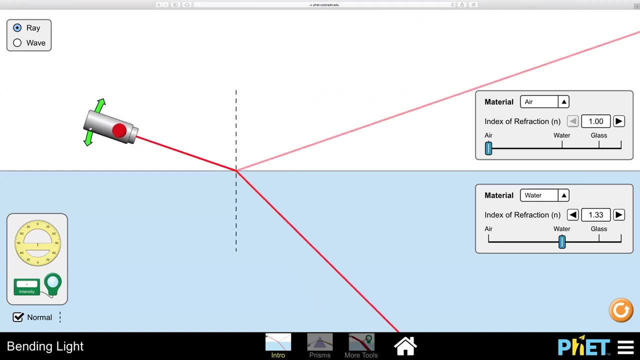 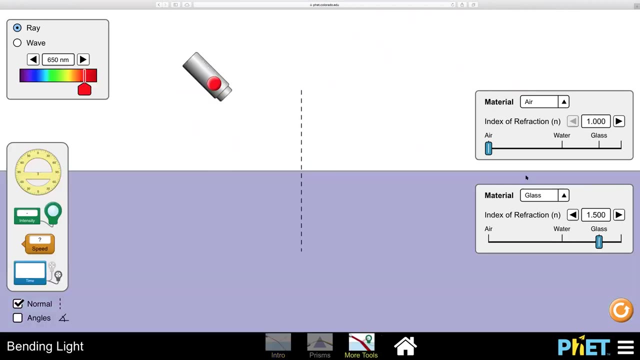 iPad and basically, here's some light and, as you can see, some of it is getting refracted and some of it is getting reflected. Let me show you another way. So we have a air and glass. So let me change this to water, so it's similar to what we. 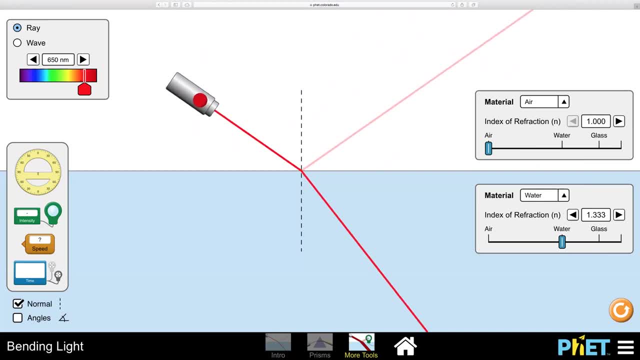 were doing before, and let's look at the angle. So my angle of incidence here is- let's make it 60 degrees, just to give it a random number. So we see that the angle of incidence is 60 and the angle of reflection is also 60.. Of course that is due to the law of reflection, But the 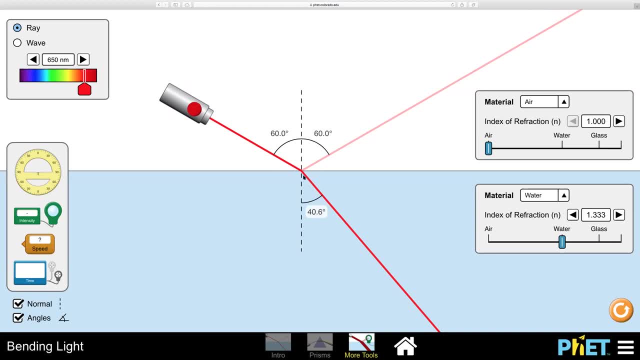 angle of refraction down here is 40.6, and again, we measure it to a line normal to the surface. So the question now becomes: okay, how do I figure out what this angle is? What equation can I use to figure that out? Now, let me keep this angle up here at 60 and let's look at 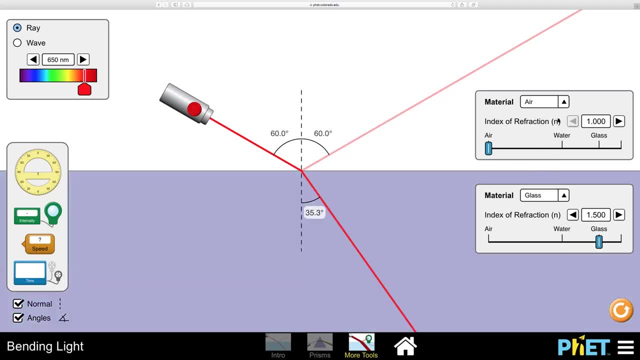 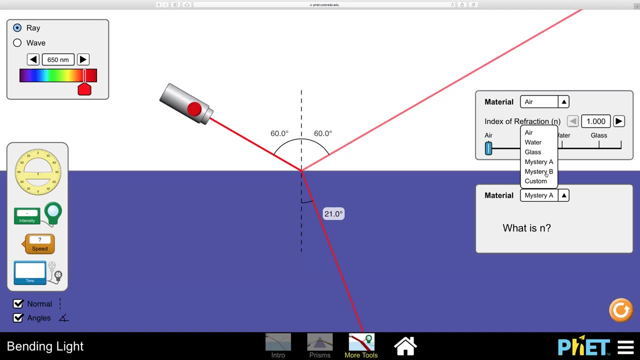 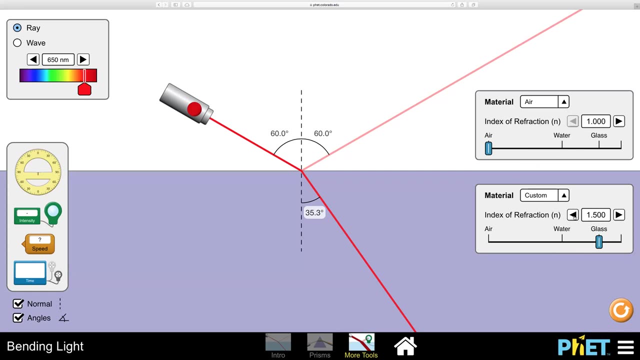 some different materials. So let's say black. Notice that the angle changed. Mystery A: angle change. Mystery B: angle change: Custom. I could change this number over here and you'll see what that means in just a little bit, But notice that if 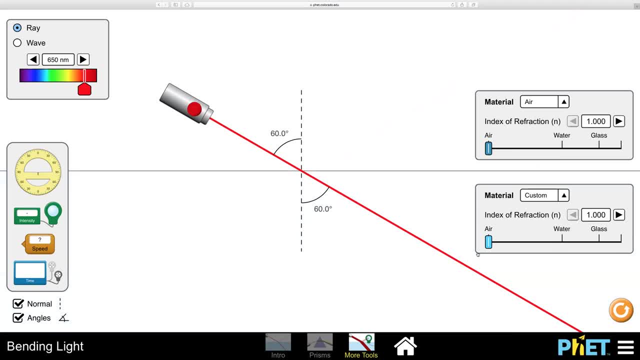 we were to make both materials air, there's a difference between the angle of refraction and the angle of reflection and the angle of refraction. And if we were to change that by a little bit just over here to the left, here there's no. 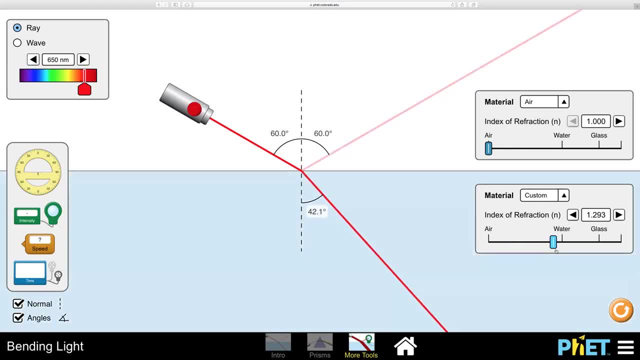 refraction happening And as we change the material right, make that index of refraction bigger and bigger and bigger we can- we could- deflect that light more and more and more and more. So the higher this number right here is, the more refraction you have happening. So let's give a definition to what this thing is. 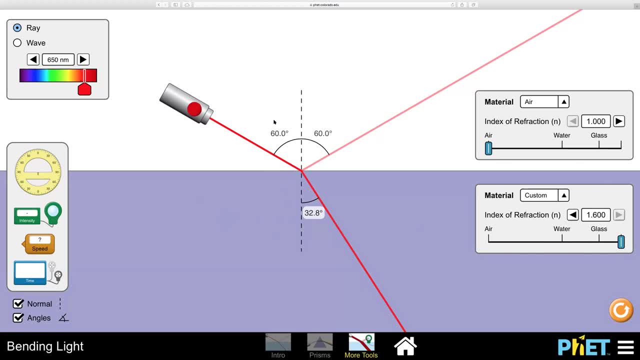 can figure out how those numbers compare for different materials. one more thing I want to show you before we get into the math is it doesn't matter what type of light it is. I'm changing the color and therefore changing the frequency and wavelength. it has no effect on the way that the light is bent and reflected in. 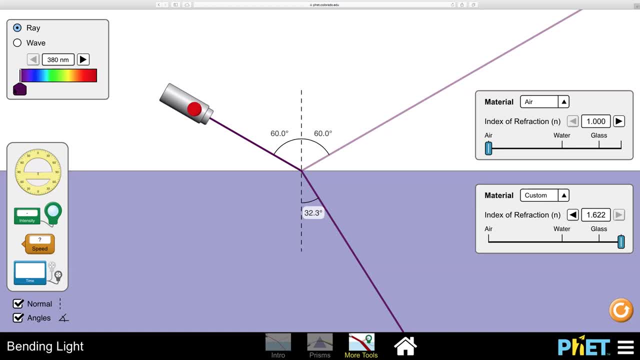 fact, if we were to take this even to a higher frequency, like UV and up, this would still happen. same thing with the other extreme, a lower frequency, infrared and lower- same thing happens. it doesn't really affect the way that light is bent. cool, now let's go back to the 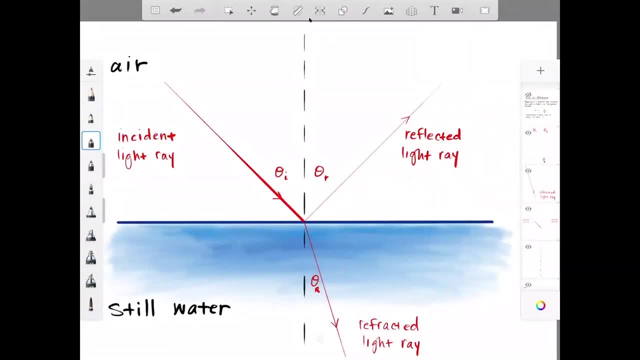 the lesson over here. so we have our incident angle, our reflected angle on a refracted angle and basically what we're going to try to figure out today is this guy right here? what is the angle of refraction? all right, let's take all this stuff off. 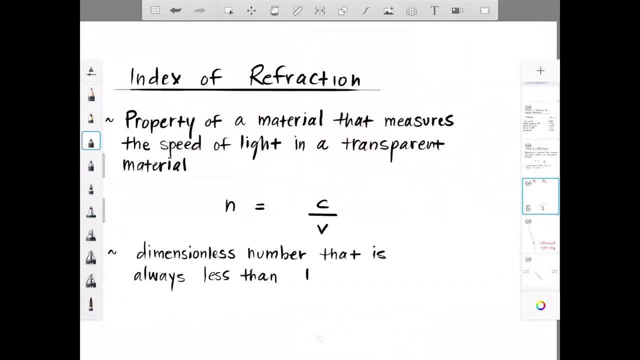 first, let's define what the index of refraction. it's a property that all transparent materials have. that is a measure of- well, it's a ratio of the speed of light over the speed of light inside of that material. so it's a speed divided by speed. 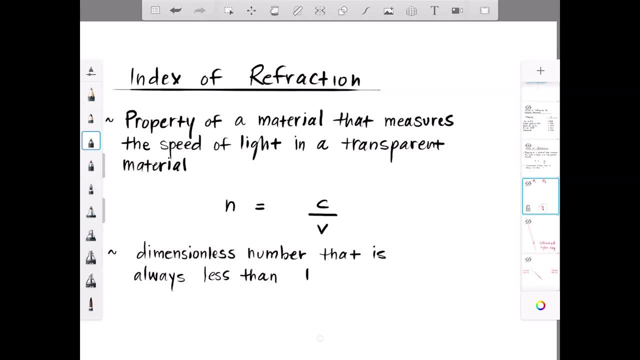 therefore, you're just going to get a number. it's dimensionless and it's always going to be a number, not less than one. I don't know why I wrote that it's actually greater than one- my mistake. it's always going to be one or bigger, if your index. 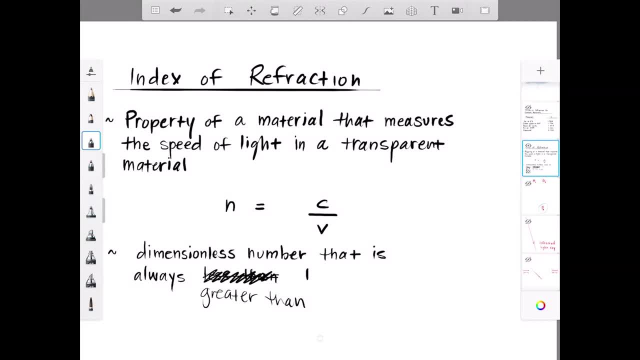 of refraction is one that means that the two materials that the that the light is traveling through are the same materials, or it could mean that there is just no refraction happening whatsoever. okay, so it has to be one or bigger. so, again, this is something that is dependent upon the material that you have. so let's look at 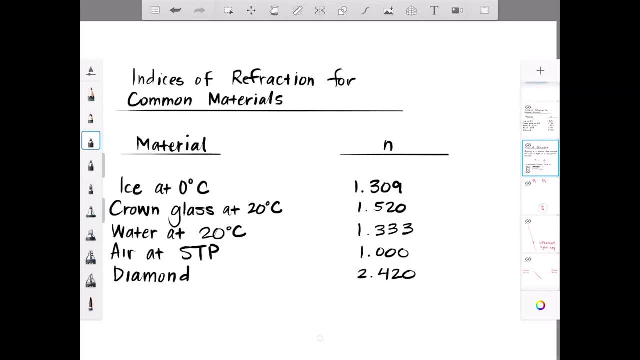 a couple of indices of refraction for different materials. now let's say you have ice at zero degrees Celsius, so, like perfectly frozen water ice, the index of refraction becomes 1.309. you have different kinds of glass, so crown glass at a standard temperature of 20 degrees Celsius, which is about 70. 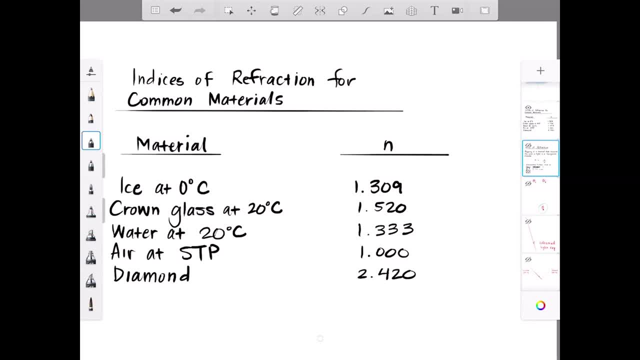 degrees Fahrenheit is 1.520. water at a standard temperature, 1.333 air at standard temperature, and pressure pressure also has an effect on this, but let's not get too into that. one point, zero, zero, zero. there's more decimals after that, but we could. 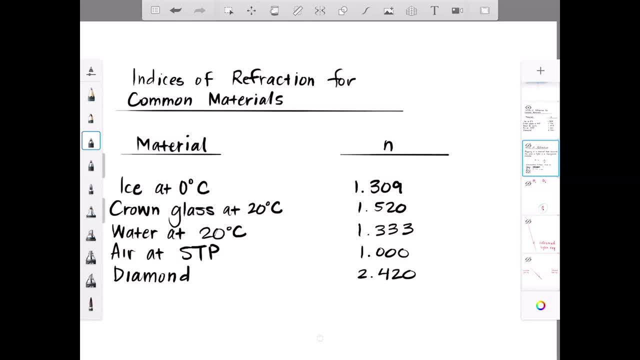 approximate it to one point zero, zero, diamond two, point four, two, and let's add one more to this, something known as the vacuum, which is literally nothing. that one is exactly one point zero, zero. we could do the same thing, but we could do the this forever, okay, but if we're talking about regular error, we could 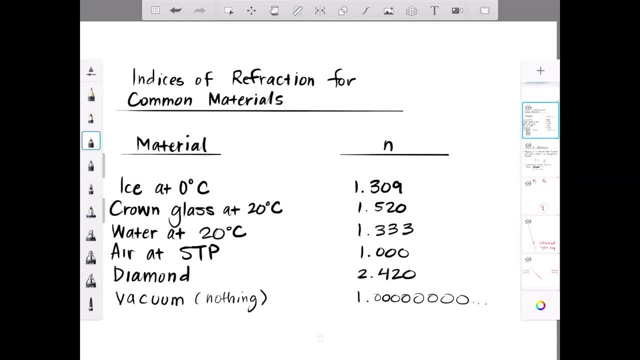 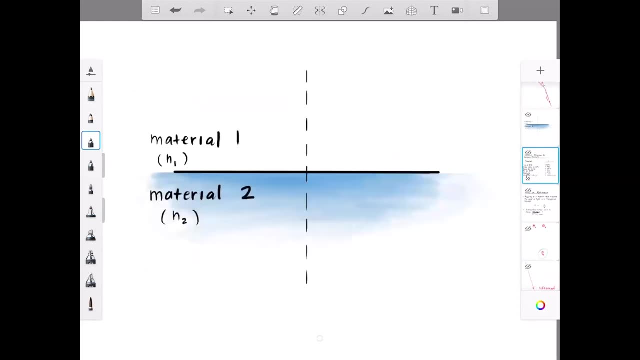 approximate it to one point, zero, zero as well. now let's look at the, at the law that dictates how this, these angles, work. okay, so let's say we have our two materials, material one and material two. each one of these guys has its own index of refraction, and one and N 2. 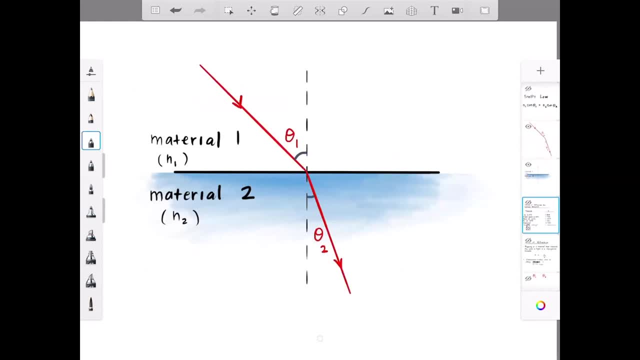 as my light ray is incident upon the material. on the second material it gets refracted, so that first angle, angle of incidence, will be what I'm going to call theta 1, and the angle of refraction would be theta 2. the formula that dictates how this behaves is known as Snell's Law, which looks like this: 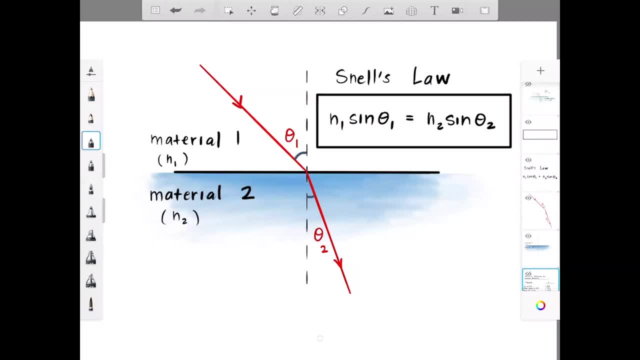 N1 sine of theta 1 equals N2 sine of theta 2.. So, using this formula, using Snell's Law, you could determine, if you knew what the angle of incidence was and if you knew the two indices of refraction, what is going to be the second angle, Another thing that you could determine. 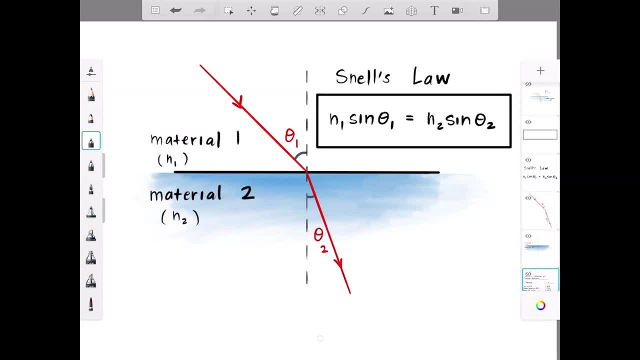 is okay, let's say we only know one index of refraction, but we know both angles. You could figure out the other index of refraction. Usually you would use it in that way because sometimes you'll be dealing with some unknown material. Okay, this is the only formula we. 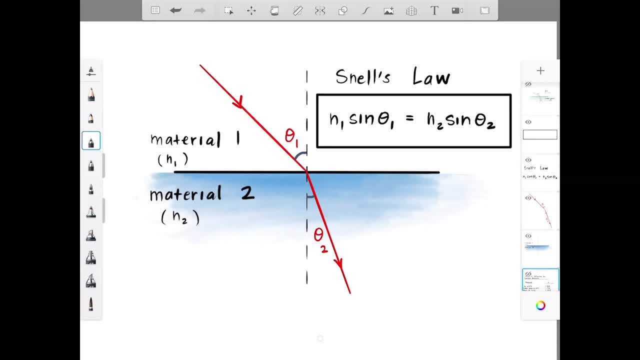 need for today's lesson. N1 sine theta 1 equals N2 sine theta 2.. So this is the only formula we need for today's lesson. N1 sine theta 1 equals N2 sine theta 2.. Let's look at some. 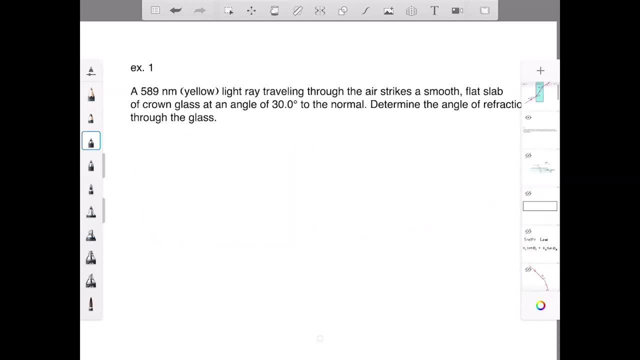 examples on how to use it. Example one: It says here: a yellow light ray traveling through the air strikes a smooth, flat slab of crown glass at an angle of 30 degrees to the normal. Determine the angle of refraction through the glass. So here is a picture of what this 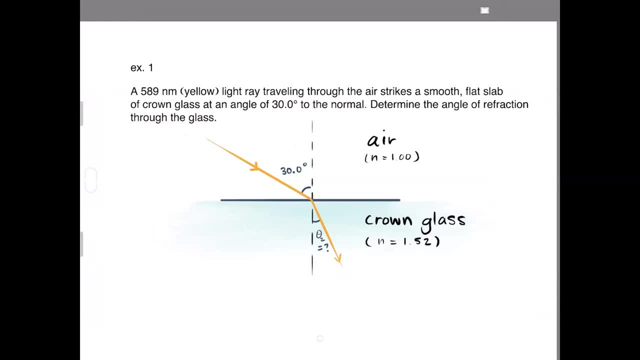 looks like You have your air. We could approximate the index of refraction to be 1.00, and the crown glass has an index of refraction of 1.52.. We know that theta 1 is 30 degrees, so we 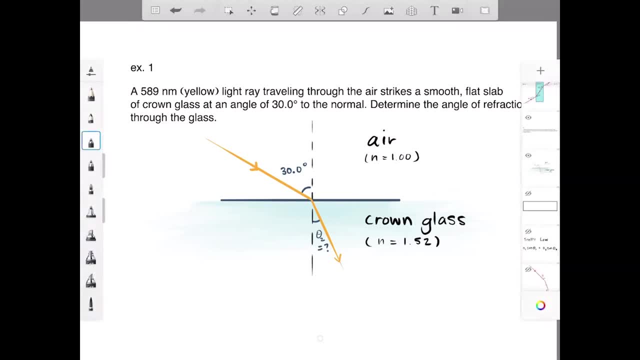 got to figure out what theta 2 is. Okay, here we go. So here's what we know Again. we know that theta 1 is 30 degrees. We know that N1 is approximately 1.00.. We know that N2. 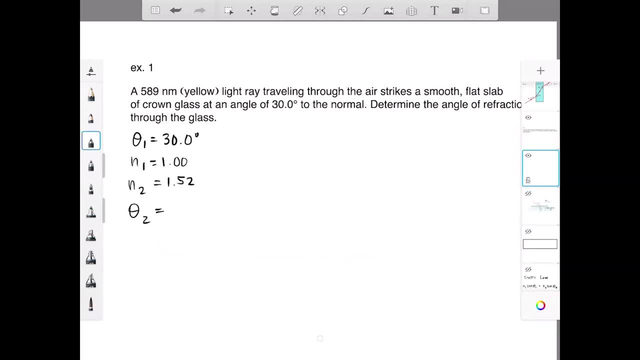 is 1.52.. We want to figure out what theta 2 is. So here's what we do, Using our formula Right: N1 sine theta 1, equals N2 sine theta 2 equals N2 sine theta. we just plug this stuff in, all right. so we got one point zero, zero times nine. 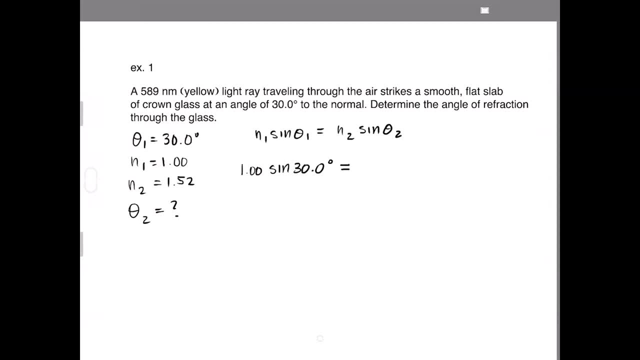 thirty equals one point fifty two sine theta two. on the left hand side we got one times sine 30 and I'm using my calculator here. it's equal to exactly point fifty. let's leave it at three, six, six, one point five, two nine theta two on 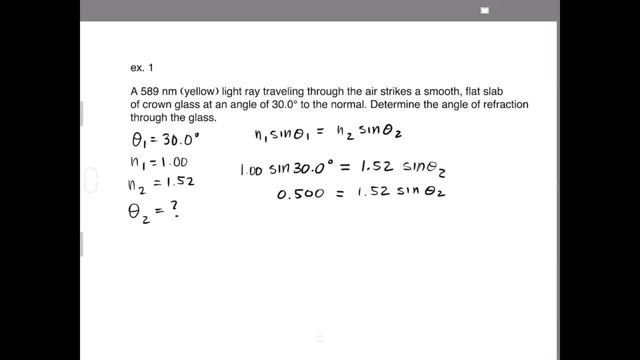 the right. my divide both sides by one point fifty two. that cancels out, and then I end up with sine of theta. two equals zero point three, two, eight, nine, and there's a few more decimals after that, but we could just leave it there, okay, so I have. let's see: one, two, three. 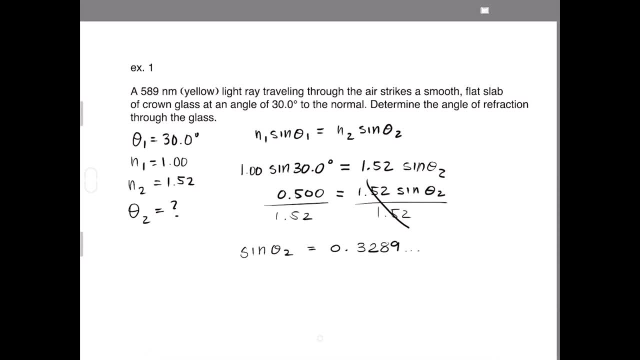 six people in here right now. out of the six of you guys in here, do any of you guys know what to do next? how? how do I get theta out of a sine theta? what should I do? you can write it in the chat if you think you know. 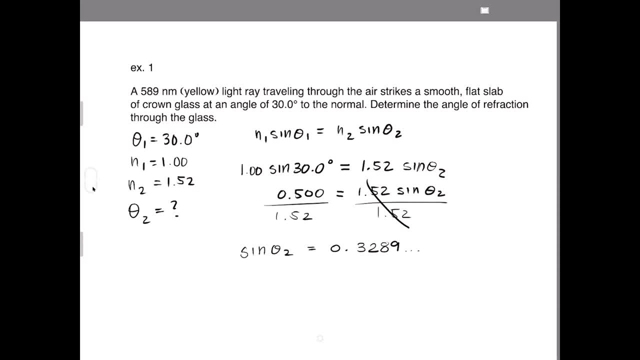 okay, what we need to do- and you can do this on your scientific calculator- is the inverse sign like this: you do it on both sides of the equation. so what ends up happening on the left-hand side when you do the inverse sign of sine? those two functions cancel each other out and you're just left with the stuff inside. 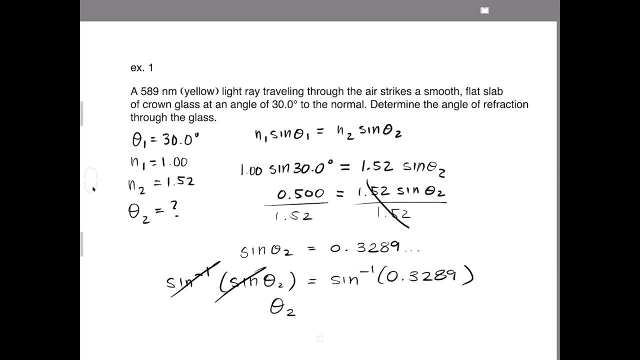 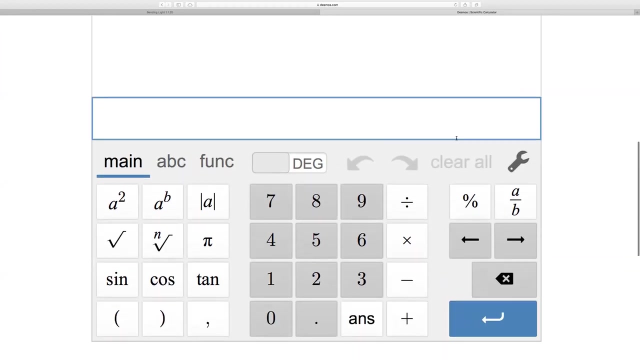 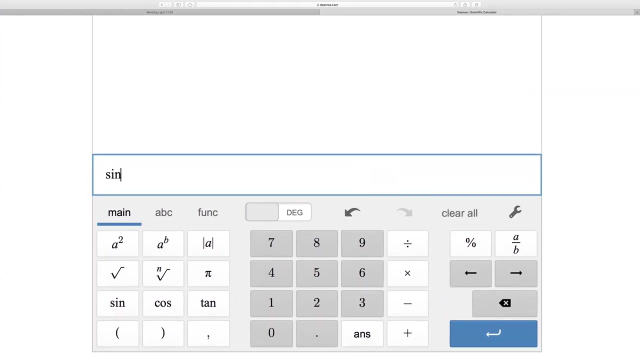 of sine, which was theta 2. now, if you're using decimals, let me let me go ahead and show you what that looks like. I'm going to share that screen with you guys as well. all right, that's really good, that's better. so you could just type in: sine minus 1. 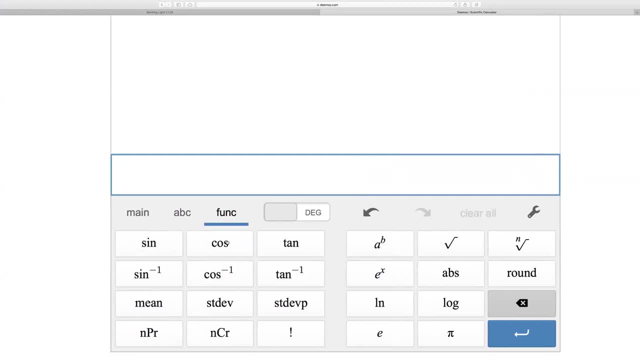 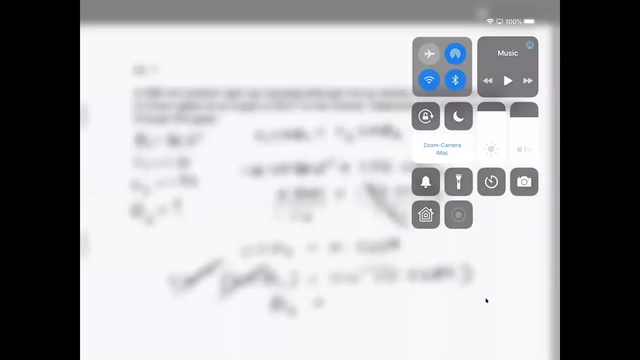 or you don't like doing that. you can go to function and then just type this one in here. so we had zero point three, 289, and there's your angle, right there. alright, let's go back to the iPad, and there you have it. the angle of refraction is: 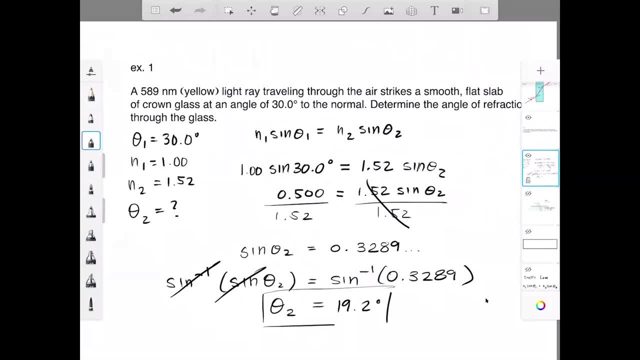 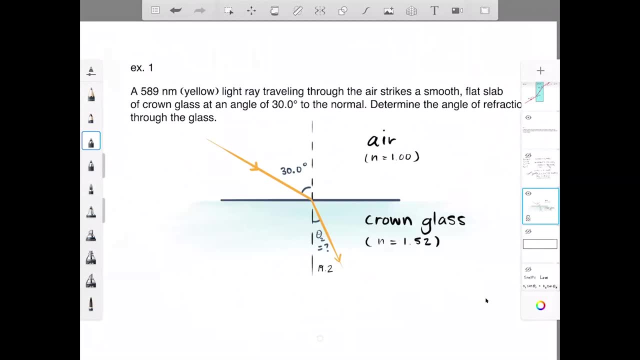 19.2 degrees. so if you go back here, this angle right here will be 19.2 degrees. so again, if you are ending up with sine of theta on one side and you want to get theta on your calculator, do sine minus one. this is known as inverse sine or arc. 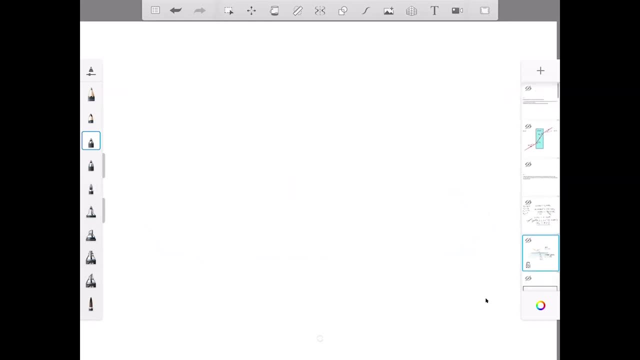 sine. all right, let's look at another example. this one's interesting because we're dealing with a different type of situation, where you have a material that is kind of sandwiched in between another material, so you have your light rake traveling through on its material. it refracts through another piece and then 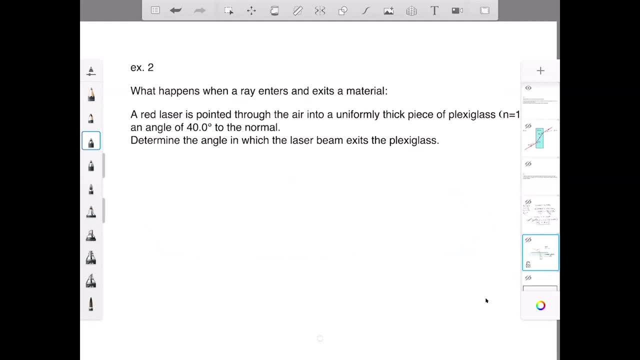 exits on the other side back into the original material. something like this for this problem: our laser is coming in at an angle that is 40 degrees to the normal. now for some reason I wrote here 30 degrees, but it's supposed to be 40 anyway. it is traveling through air. it hits this plexiglass which has an index. 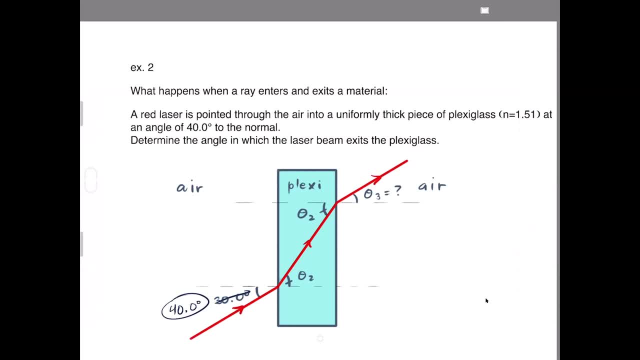 of refraction of 1.51, and then it exits at the air at some unknown angle. now there's an easy way of doing this and there's a harder way of doing this. the easy way is to use geometry and symmetry for this problem, just to get a sense of. 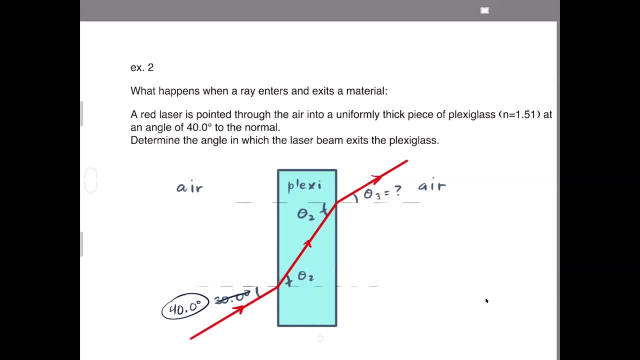 how the light rake is and how the whole structure is going to affect the light rake. If we have a uniformly thick piece of glass right, as you see right there in the middle, we know that this theta 2 over here and this one have to be the same, because it's like 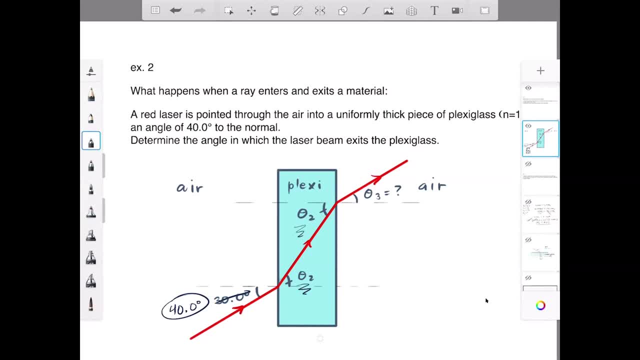 taking a rectangle and then drawing a diagonal line across. The two triangles that form as a result of that are, of course, congruent to each other. We know that from geometry, So we can reasonably suspect that this angle and this angle will end up being the same. 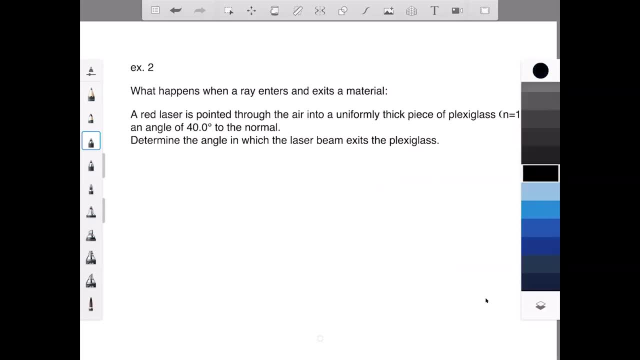 Let's go ahead and prove that Now. let's say: okay, so we started with n. we started with: n1 equals approximately 1.00,. n2 equals 1.51,. theta1 equals 40 degrees. theta2 equals we. 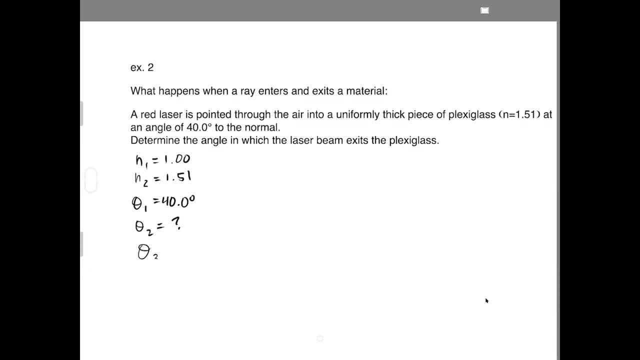 don't know, but that doesn't matter, because what we need is theta3.. So we're going to have to figure out what theta2 is as an intermediate step, so that we could then apply the same rule to theta2.. All right, so let's go ahead and do the same thing that we did before: 1.00 sine 40 equals. 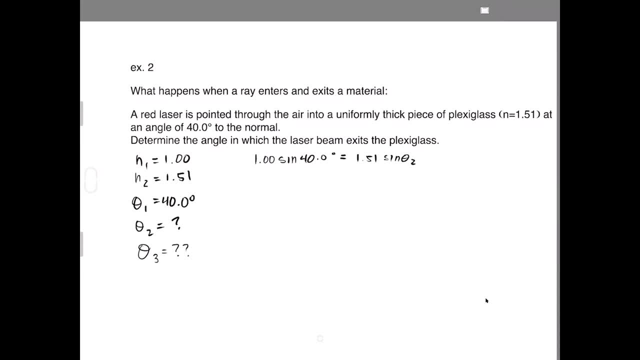 1.51 sine theta2.. One times sine 40 gives me 0.642.. Okay, So 1.00 times theta2 equals 0.8, approximately 1.51 sine theta2, divide both sides by 1.51,. 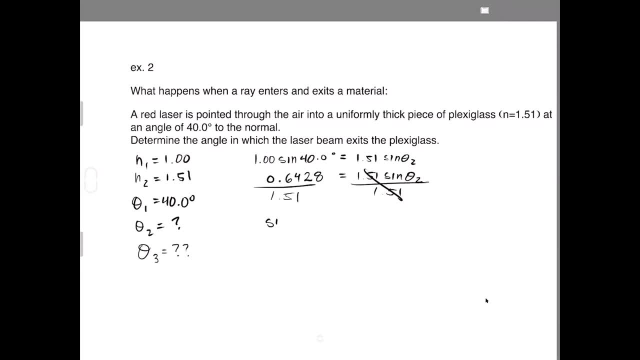 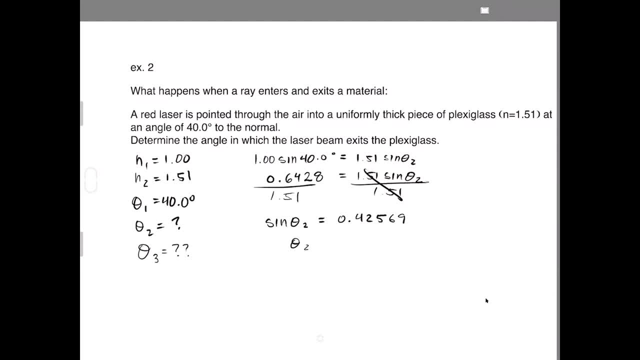 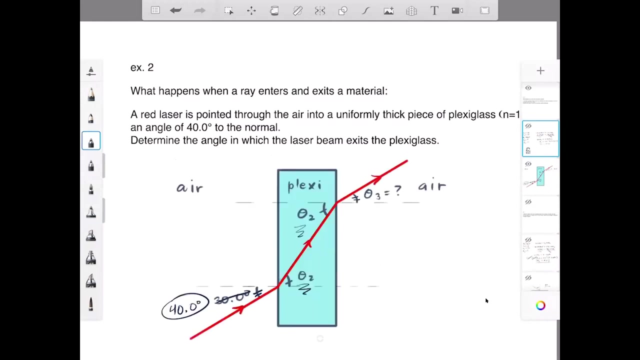 Bye. Theta. 2 ends up being the inverse sign of that number. So according to my calculator, that is 25.2 degrees. So let's keep that answer in mind. for now, Let's erase this and go back here. We now know that this angle is 25.2 degrees and this one is 25.2 degrees as well. 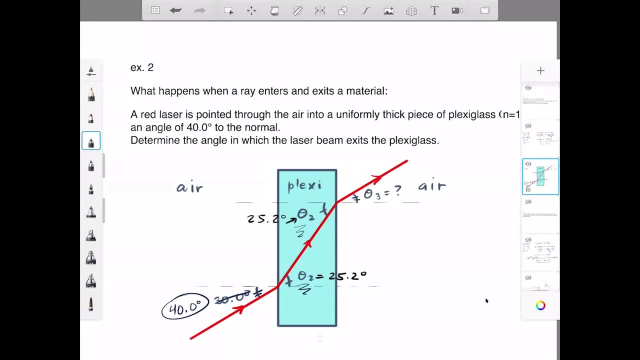 This is going to end up being your angle of incidence through the plexiglass, and this, right here, is your angle of refraction that we're going to need. So the way that we're going to figure this out is to just apply the rule one more time. 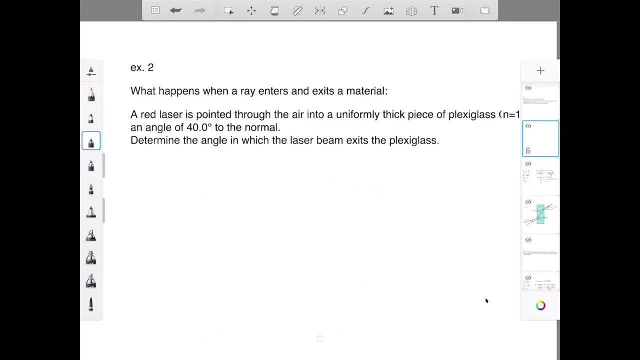 Let's go back here. So 1.51 sine of 25.2 degrees, That's 25.2 degrees. 25.2 degrees equals 1.00 sine theta 3. We're able to do this because we go back to the picture over here. 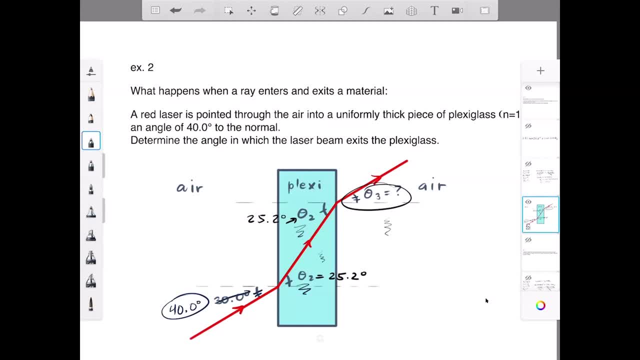 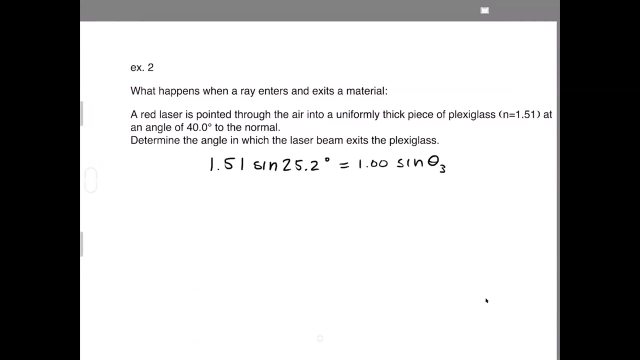 Over here we're going to have our first material, and over here we're going to have our second material, our incident and our refractive. Okay, The incident material has an index of refraction of 1.51.. All right, So we're going to go ahead and apply the same thing. 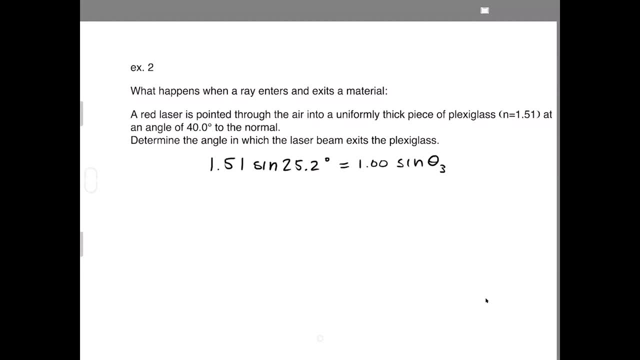 1.51 times sine of 25.2 is 0.6427.. Okay, Okay, All right, We're going to do the same thing And I'm just going to use my calculator to see if I can do that right away. 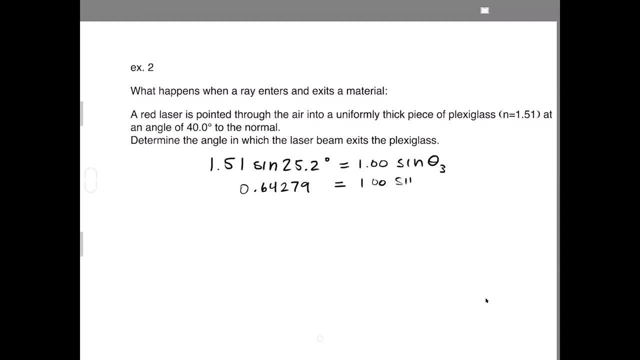 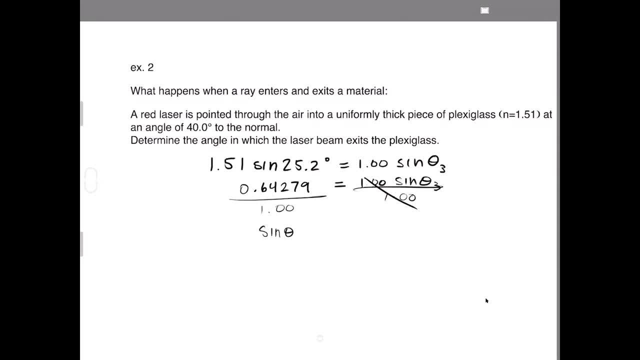 1.51.. 1.51.. 1.51.. 1.51. 1.51.. Yeah, 64279.. 1.00, sine theta. 3.. 0.64279 do the inverse sign of that number. 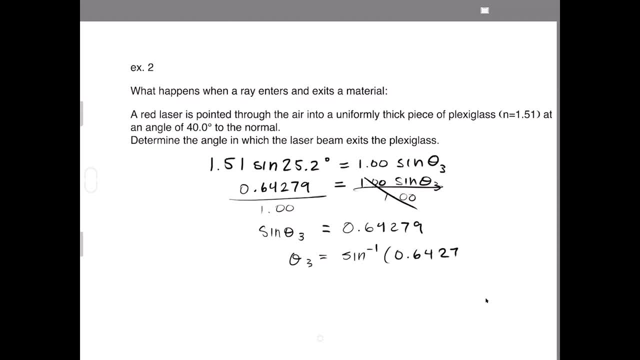 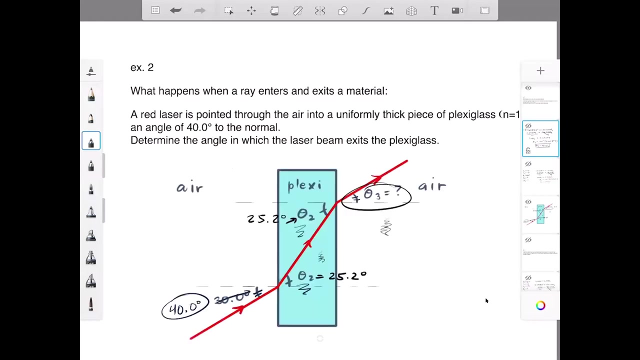 and then we have a curious result here: beta 3 is equal to 40.0 degrees 0.64279. now that ends up being exactly equal to the angle that the um that the light ray started with. so if we go back to the picture, one of 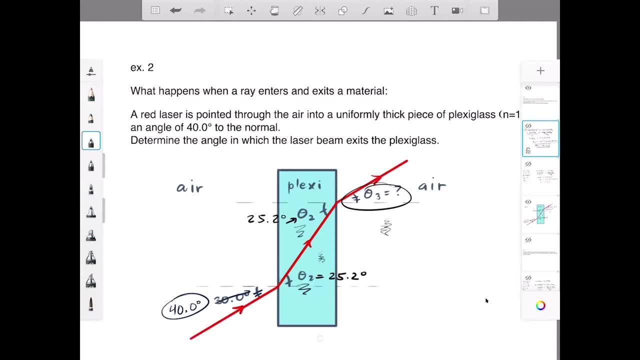 the predictions that i made was like: okay, i think, due to the symmetry, due to the geometry, i think that theta 3 will be exactly equal to theta 1, and now we see, through snell's law, that this is, of course, true. so here, allow me to make a statement. uh, let me erase all this. 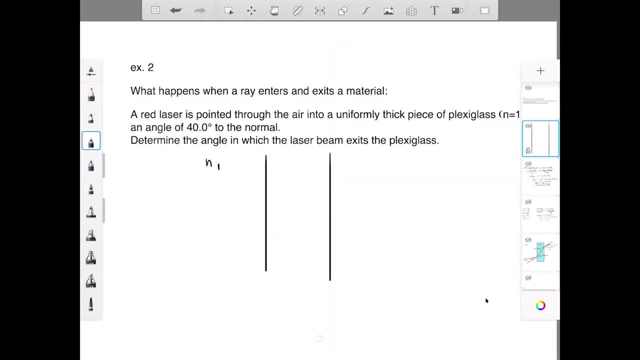 so let's say we have um and one and two and then and one again. right, what's going to end up happening? we have our light ray. we have a- let me put it down here our light ray. sorry guys, i'm having an issue here. Here's our light ray. it's going to diffract like that. 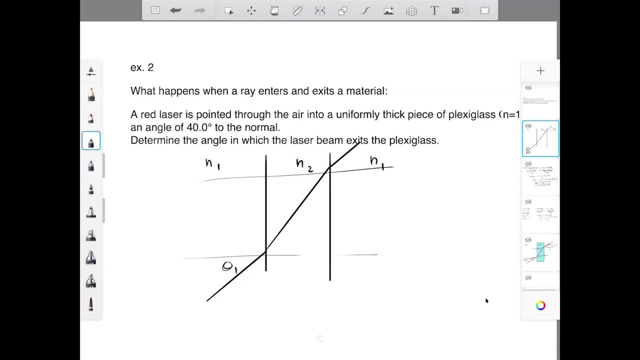 So let's say that this is your angle of incidence. here's your angle of refraction. this one is going to be the same and this one is going to be your new angle. If the materials on the left and right are the same material, then theta one is going. 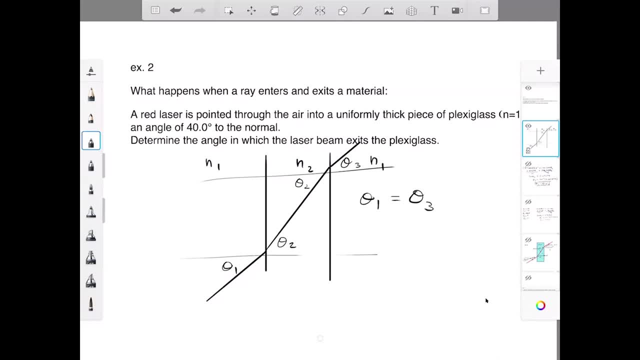 to be equal to theta three. We just proved that using Snell's law. And let me make one more statement. Let's say we have three different materials: N1,, N2, and N3.. This is going to be a little bit different. 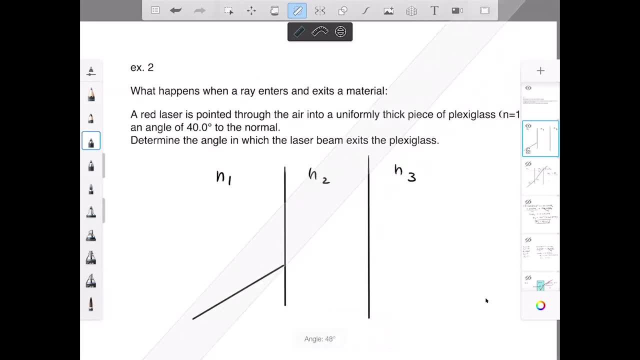 Here's your incident light ray. it's going to refract a little bit, Okay, And then it's going to refract again at some other angle that we don't know. The way we work this one out is like this: Here's r theta one- r theta two. these two, of course, have to necessarily be the same. 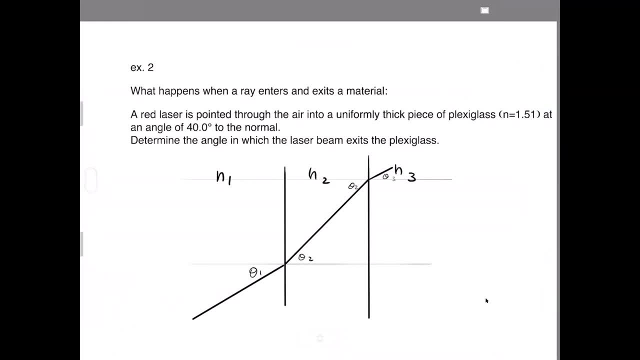 and then here's r theta three, Okay, Okay. So if you have three different materials and a situation like this, you could imagine it's like going through air, then going through water and then going through glass, Right, Actually, no, it makes more sense to say water through glass than through air. 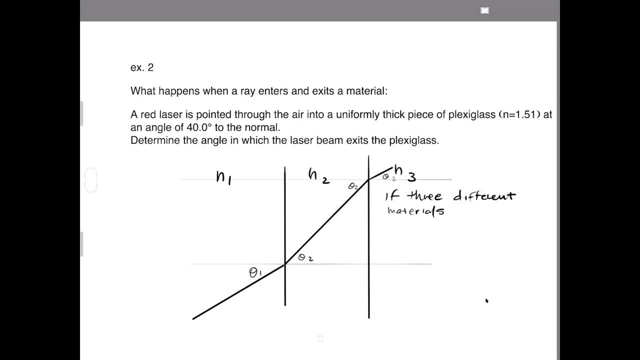 Like. imagine having a glass of water sitting on your table. the light ray that's hitting the glass, It's going through the air and then it refracts through the glass and then refracts even further through the water. right, Use Snell's law three times. 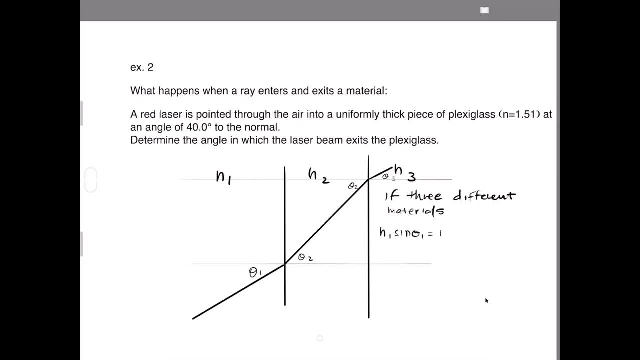 N1 sine theta one equals N2 sine theta two, which is going to be even further equal to N3 sine of theta three. Okay, So you could use any of these equal to each other. You could say: N1 sine theta one equals N2 sine theta two. 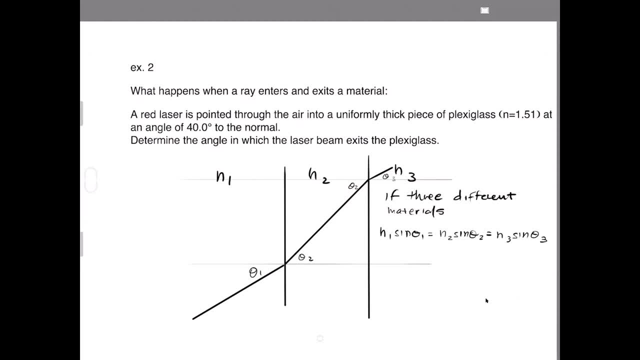 You could say: N1 sine theta one equals N3 sine theta three. Or you could say something like N2 sine theta two equals N3 sine theta three. Think of it like A, B and C right A equals B equals C. If A is equal to B, then A equals B. 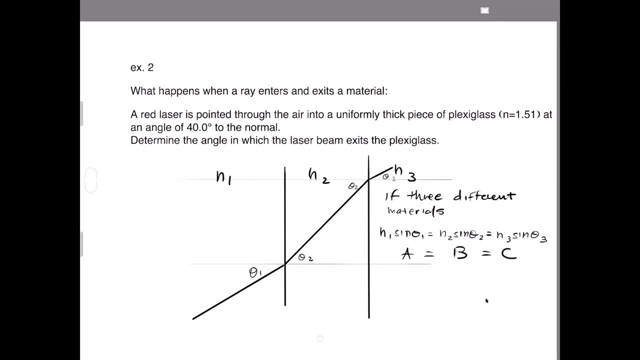 Okay, Okay, Okay, Okay, Okay, Okay, Okay. If A is equal to B, then…. and B is equal to C, then A is equal to C as well. These are the transitive properties, of course, in math. 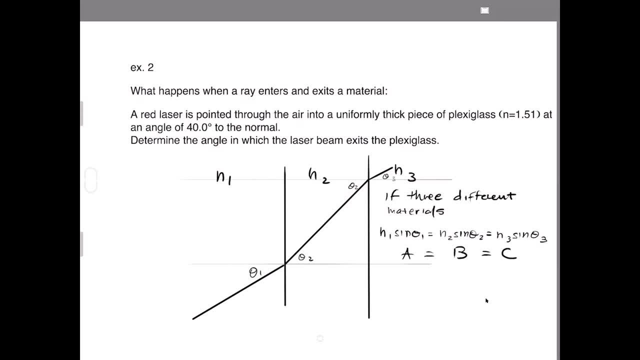 So there's going to be a question like this on the homework as well. There isn't really a point for me to show you an example of doing this, because it's the same math, But just know that if you have three different materials, you could use the Snell's law equation. 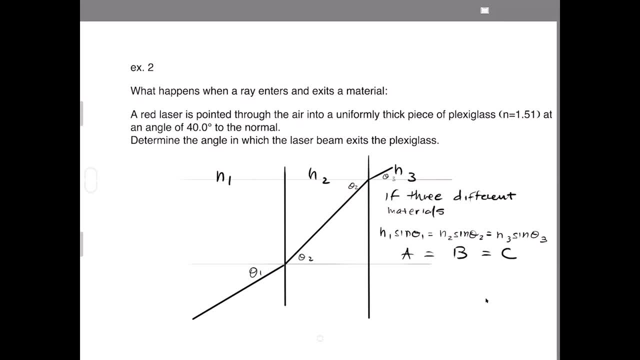 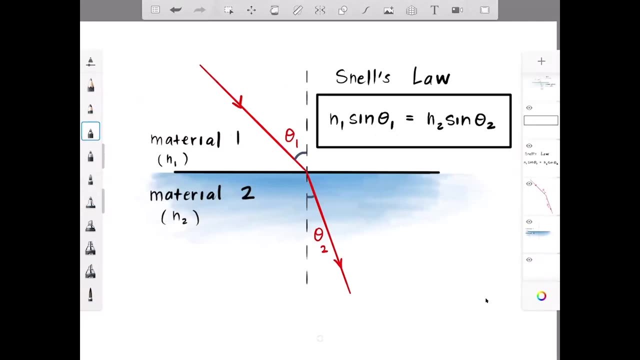 in this way. Okay, and that is it for me today. so just to recap what we talked about, let me go back to the other slide. snell's law is the equation that dictates how a material refracts through some other material. um, it is the formula, and one sine theta one. 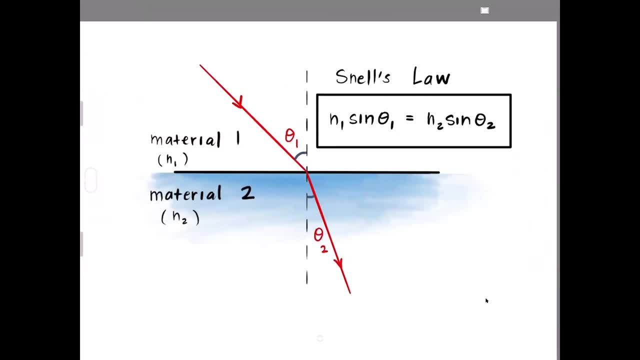 theta one equals n two sine theta two. where n one is the index of refraction of the first material, theta one is the angle of incidence, n two is the index of refraction of the second material and theta two is the angle of refraction when you have more than two materials, three or more. 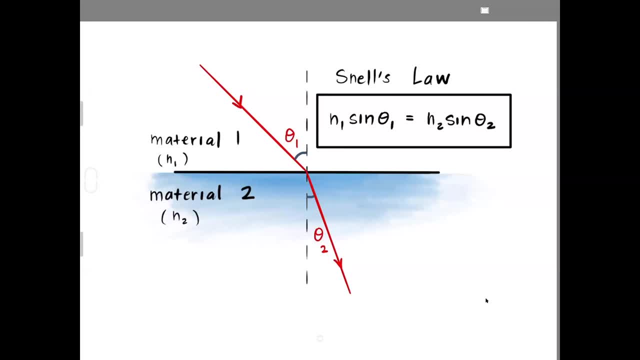 you could just continue adding equal signs to this. so let's say you have three materials sine theta one equals n two. sine theta two equals n. three sine theta three, and you could add more and more, as many as you need um for the homework that you're going to see when we 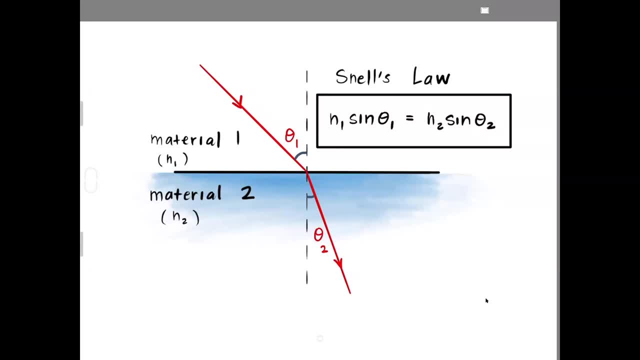 get off the call, there will be one problem dealing with three materials. the rest of them only deal with two materials. all of the indices of refraction will be given to you in the homeworks and the angles, of course, will be given to you as well. so having said all that, let me stop the screen share. let me also. 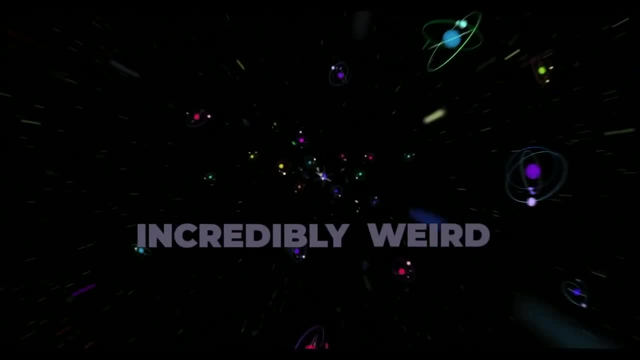 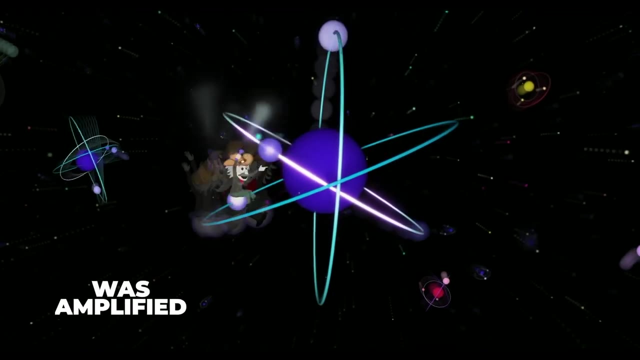 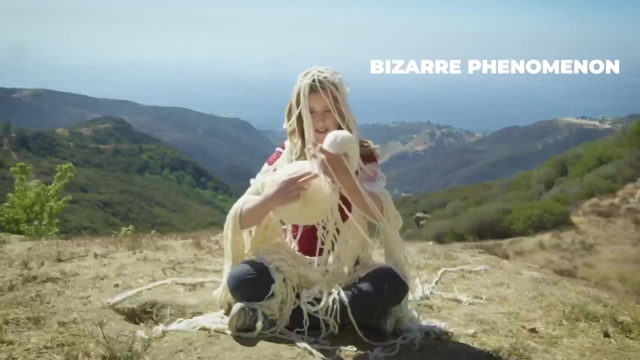 The universe has always been an incredibly weird place, and when scientists finally unlocked the world of quantum mechanics, that strangeness was amplified many times over, From the discovery of particles being a particle and a wave at the same time, to the bizarre phenomenon of quantum. 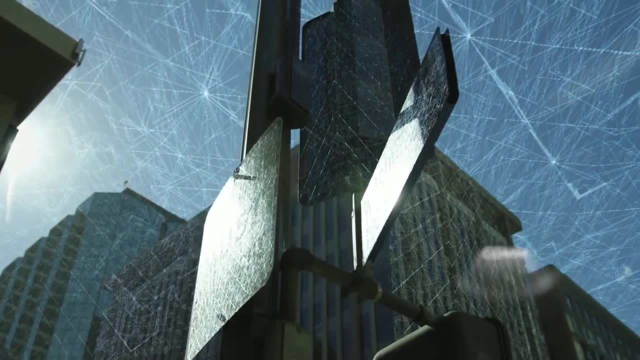 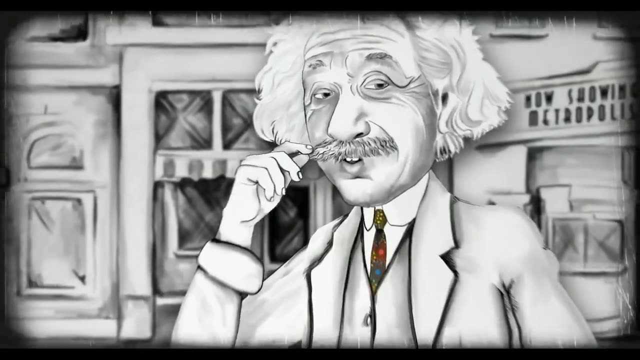 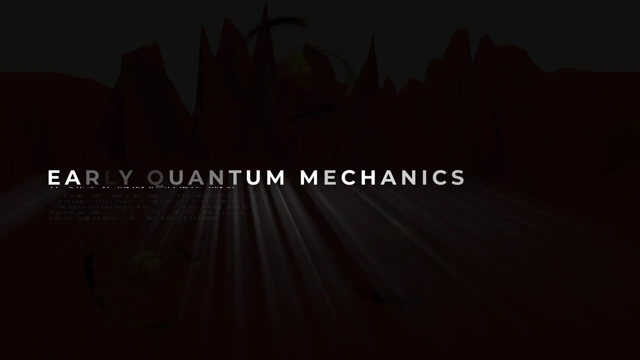 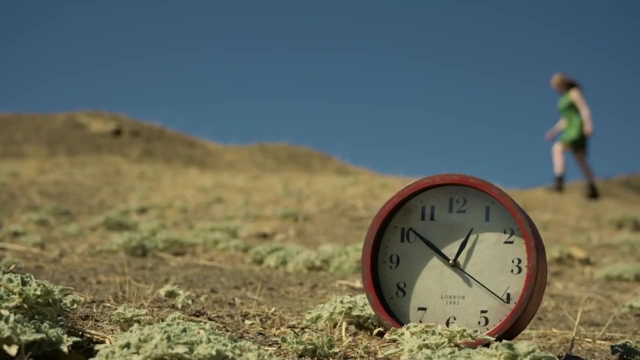 entanglement. the world of the very small seems to violate the common sense and logic that dominated science from its founding. Today we're diving into the wacky realm of quantum mysteries to uncover the reality of quantum superposition. Early Quantum Mechanics Before the 1920s, many scientists in the physics field believed that they may be closing in on. 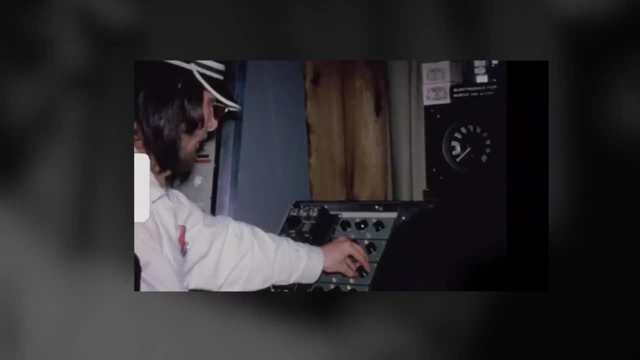 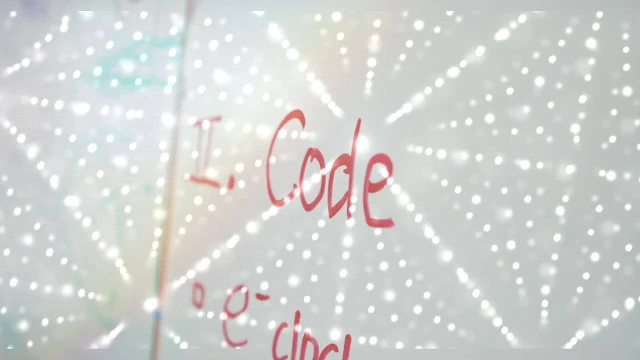 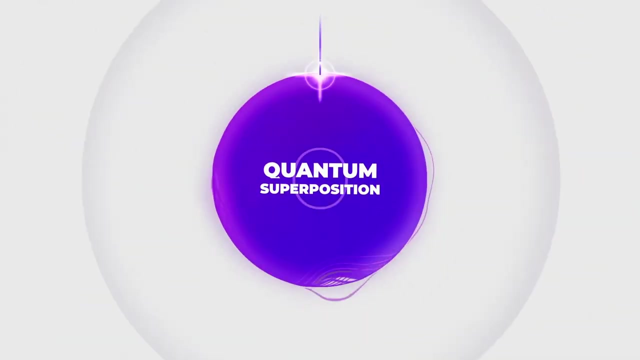 understanding the vast majority of our reality. But then new experiments probing into the bizarre world of subatomic particles opened the door in the weird and crazy world of quantum mechanics. There were many new concepts, such as the incredible phenomenon of quantum superposition. 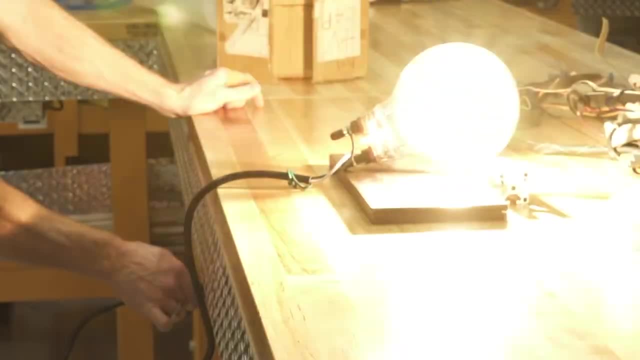 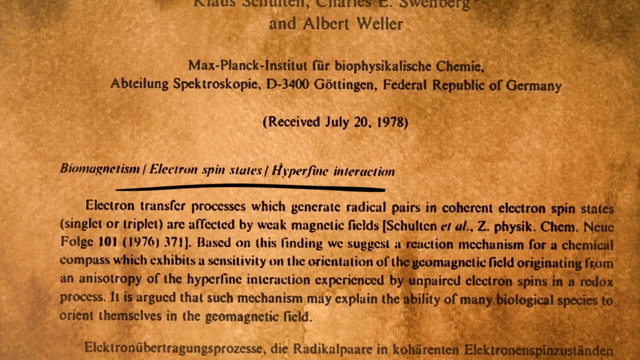 With this new form of physics came a huge outpour of experiments and theories that seemed almost magical. at the time. There was a rush to try and form some kind of understanding about this mysterious new realm and unlock the potential hiding inside, On the other side of the scientific 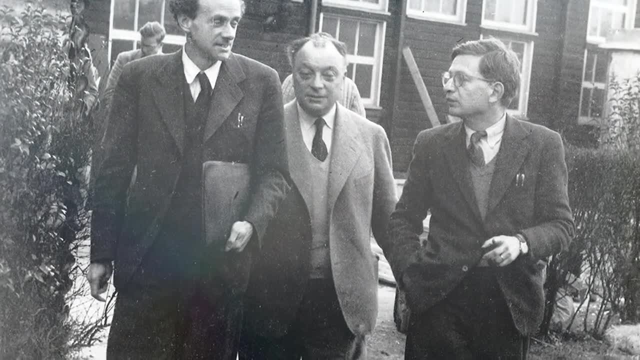 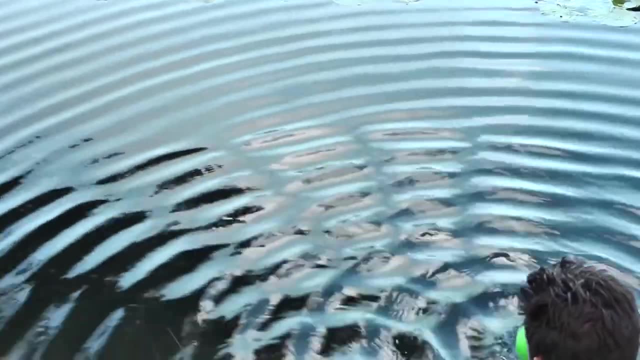 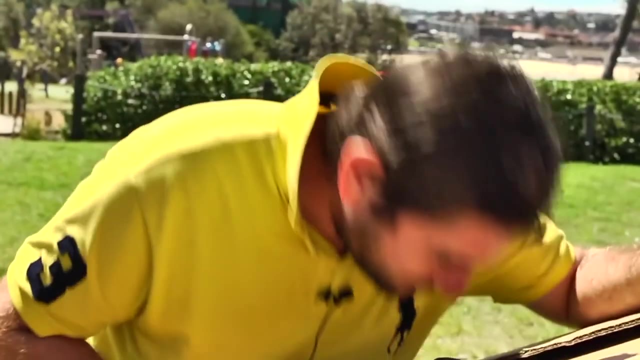 community. many of them felt uneasy about this whole new realm of reality and spent their time trying to disperse the mystery of quantum superposition. This was the first time that scientists proved the seemingly impossible realities that make up the quantum world. The nuisance of quantum science will always come out on top, but experimental findings will always come out on top and, after rigorous testing, there is no doubt that this strangeness is actually real. 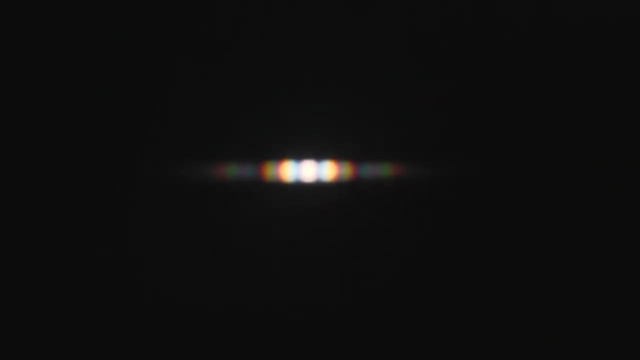 I can see tons of dots- now, not tons, but I can see dots spreading across that way Either side. Yeah, definitely, Isn't that amazing? Yeah, that's incredible. And that's just nothing else apart from two slits.